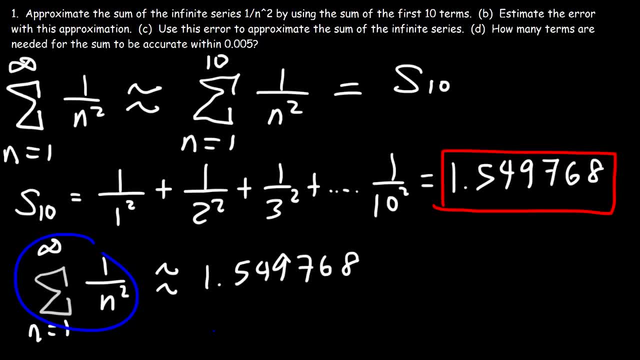 Now, granted, the true answer is going to be different than that answer, but this is simply an approximation using the first 10 terms according to part 8.. So this is the answer for part 8.. Now let's move on to part B. Estimate the error with this approximation. So how can? 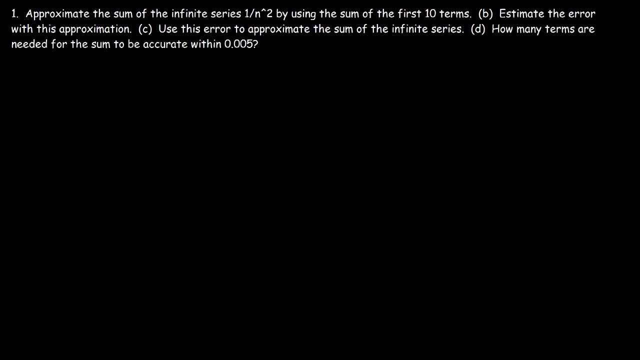 we do that. Well, let's talk about the remainder estimate for the integral tests. So let's say, if we have the sequence a sub n and it's equal to f of n, The function f has to be continuous positive and decreasing everywhere where. 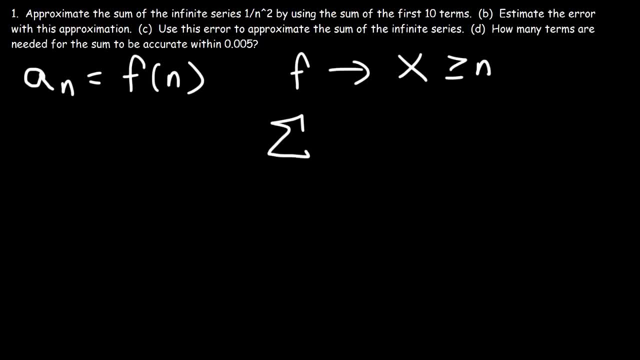 x is equal to or greater than n and at the same time, the series must be convergent. So let's check to see if these four conditions are met. Looking at the series 1 over n, squared according to the p-series, it's convergent. 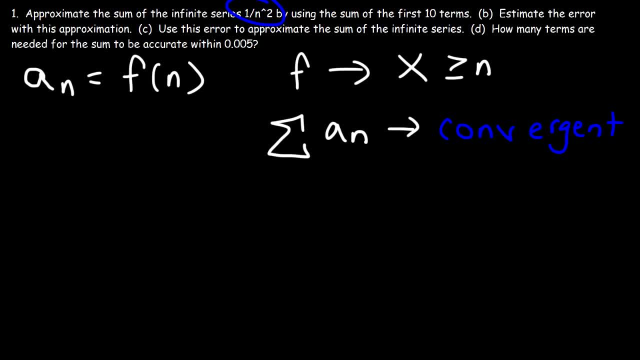 p is 2.. Anytime p is greater than 1, the series will converge. Now let's write the corresponding function. F of x is 1 over x squared. Now let's get your graph for this function, And so it's going to look like this: 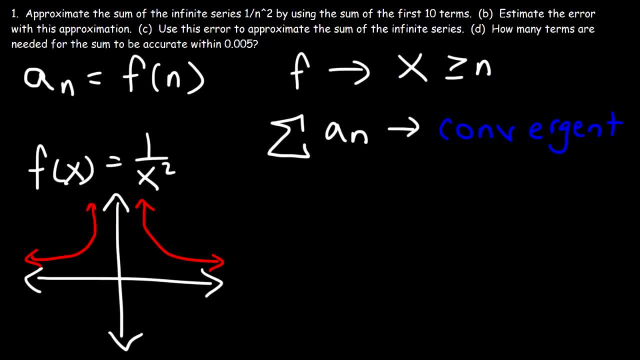 Now x has to be greater than or equal to n, And in this problem n is 10.. So we're concerned with this area of the graph. So notice that in this region the function is positive because it's above the x-axis. 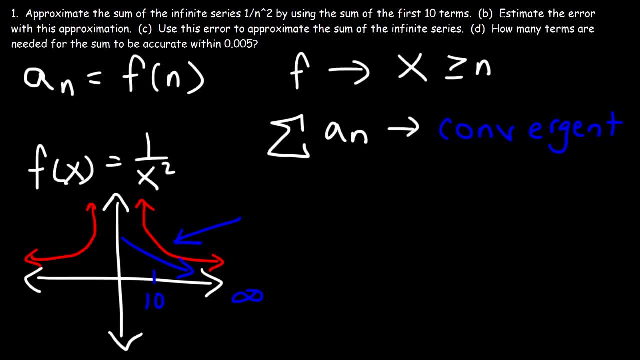 It's decreasing. We can see that it's going down And at the same time it's continuous from 10 to infinity. There's no holes, no jump discontinuities or infinite discontinuities in this region. So the criteria for the remainder estimate theorem has been met. 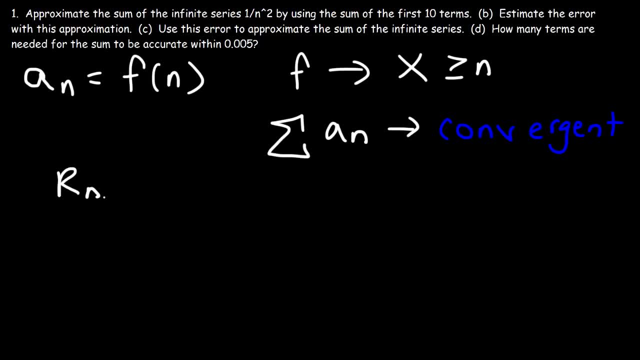 Now let's say that the remainder r sub n, is the difference between the infinite sum and the partial sum, Then this will be true: r sub n is going to be between these two integrals. So how can we determine r sub n in this problem? 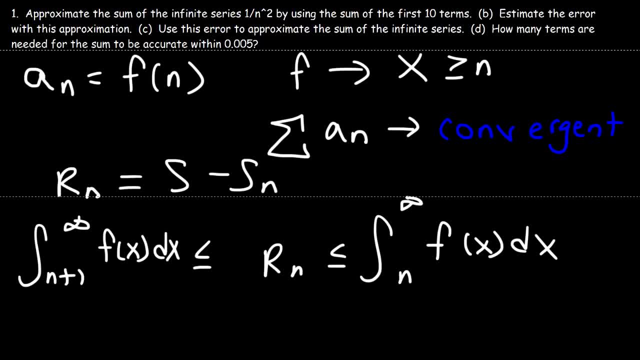 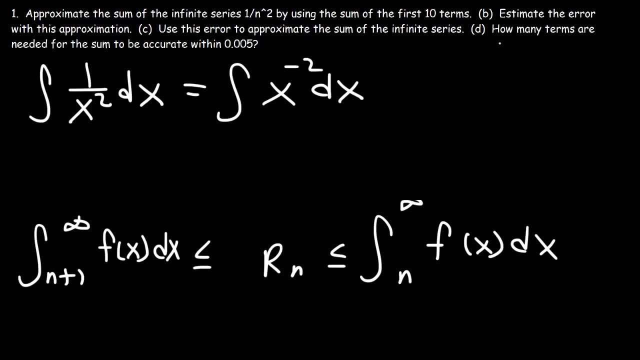 Well, first let's find the antiderivative of f of x. So f of x is 1 over x squared, And let's rewrite that as x to the negative 2.. So using the power rule, this is going to be negative 2 plus 1.. 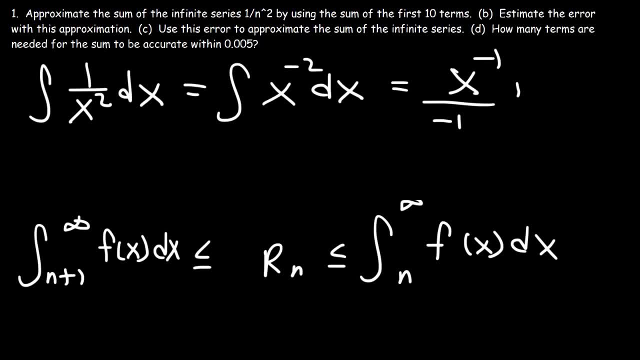 That's negative 1 divided by negative 1.. And then we can rewrite that as negative 1.. So negative 1 over x. Now let's determine the definite integral from n to infinity of f, of x, dx. So that's going to be the limit as b approaches infinity. 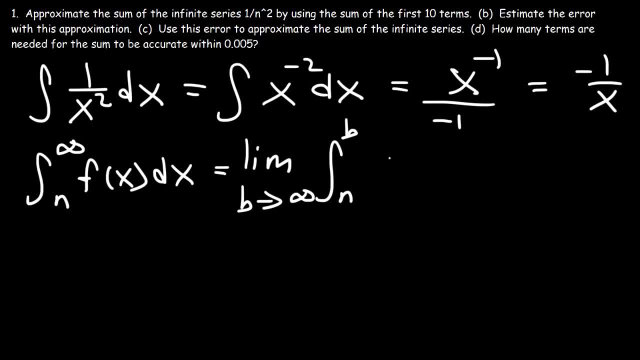 The integral of n to b: 1 over x squared dx. So that's equal to the limit as b approaches infinity. And then we know the antiderivative of 1 over x squared: That's negative 1 over x. So this is going to be negative 1 over x, evaluated from n to b. 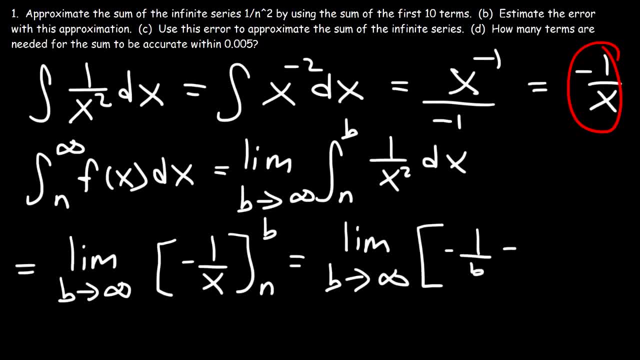 So then this is going to be negative 1 over b and then minus. Now we need to plug in n- negative 1 over n, But these two negative signs will cancel, so it's going to be plus 1 over n. 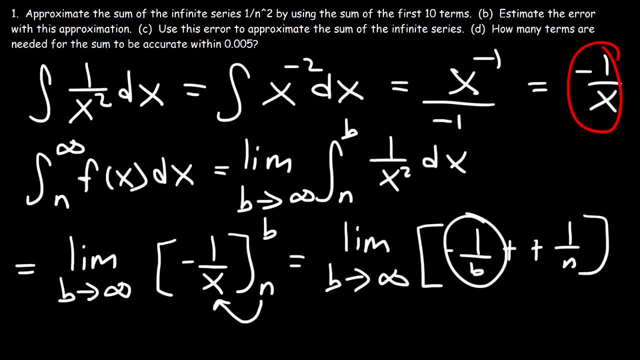 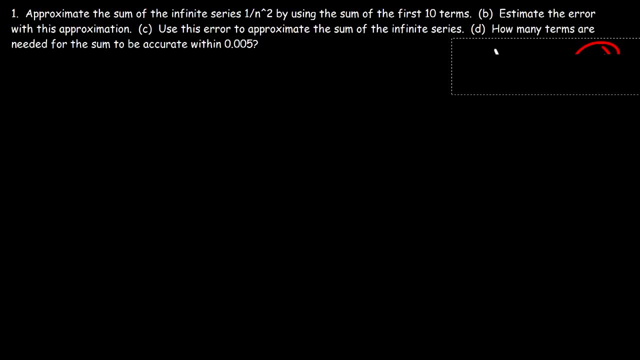 Now, as b approaches infinity, negative 1 over b Will become 0. So this is going to be 0 plus 1 over n, which is 1 over n. So let's write out what this means. So this means that the integral from n to infinity of f, of x, dx, is 1 over n. 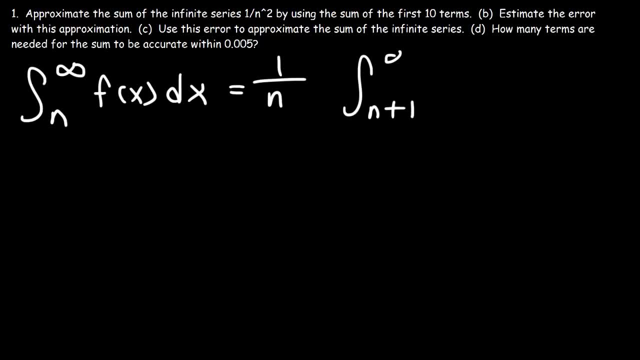 And the integral from n plus 1 to infinity. if we multiply this, we get x. you follow the same process. should be 1 over n plus 1.. Now, earlier we said that r sub n. the remainder estimate is between these two integrals. 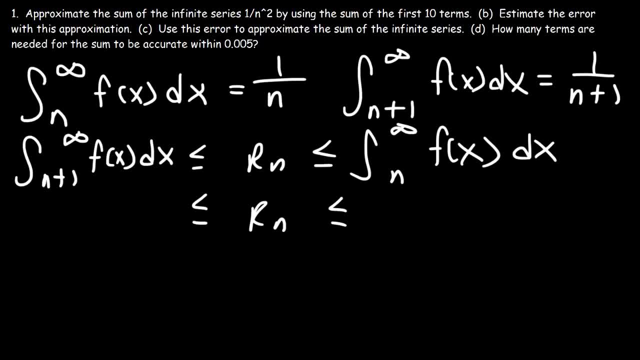 So therefore r sub n has to be between 1 over n and 1 over n plus 1.. So r sub 10 is going to be between 1 over 10 and 1 over 10 plus 1 or 1 over 11.. 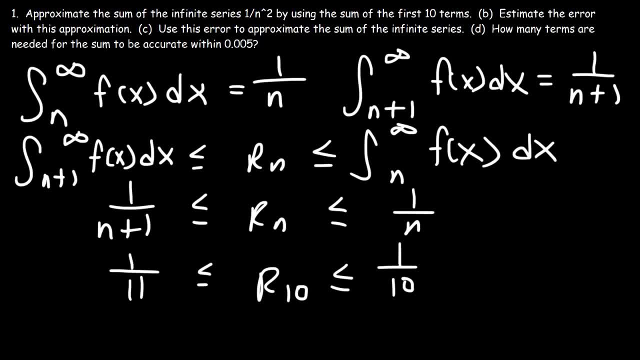 Now let's get the decimal values for this. So 1 over 11, that's going to be 0.09091.. And 1 over 10 is just 0.1.. So the remainder estimate is between these two values. 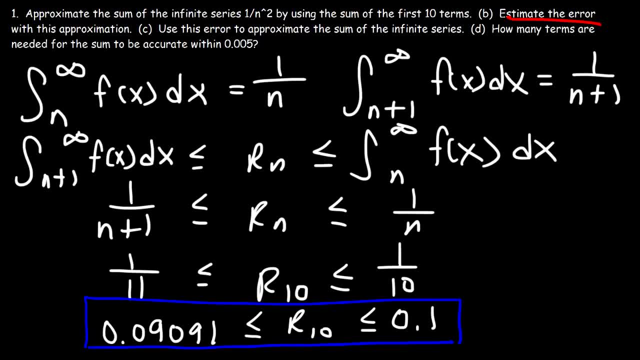 So the answer is 0.09091.. So the answer is 0.09091.. So the answer for part B estimate the error with this approximation. So we could say that the error is at most 0.1.. It's not going to be higher than 0.1.. 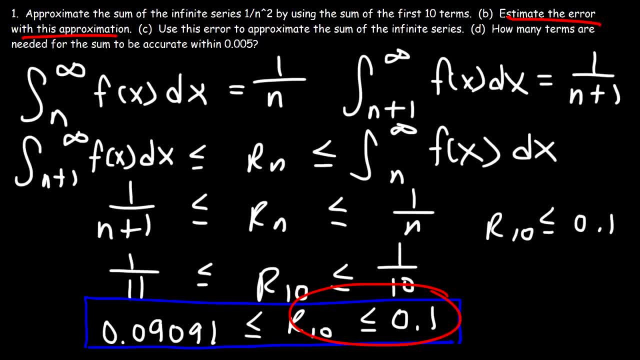 It's going to be less than or equal to 0.1.. But it's going to be greater than or equal to 0.09091.. So it's between these two numbers. Now let's move on to part C. Use this error to approximate the sum of the infinite series. 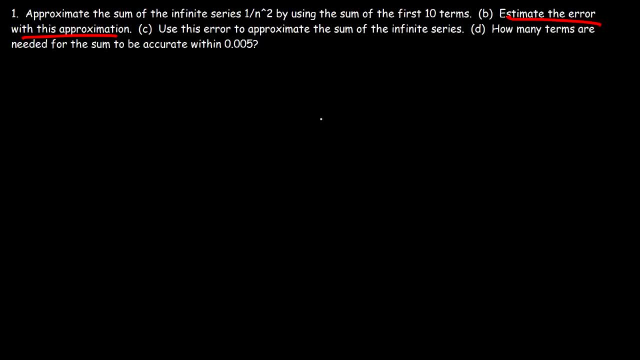 So how can we do that? So recall that early in the video we said that the remainder estimate is the difference between s and s sub n. Now it's important to understand that s is the sum of the infinite series, So it's the limit, as n approaches infinity, of s sub n. 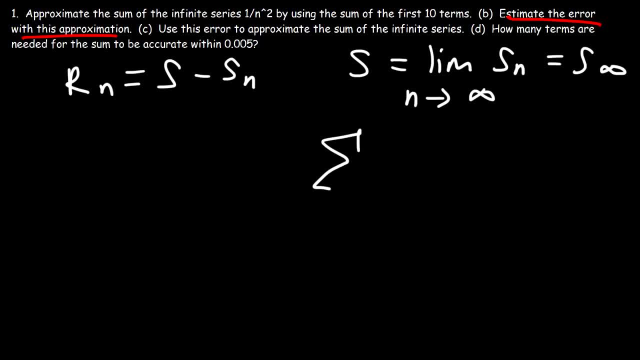 which is basically s sub infinity. So if you write a list of all the terms and you add the first term plus the second term all the way to infinity, this will equal s. We want to get a better approximation of this value. S can be approximated by s sub 10.. 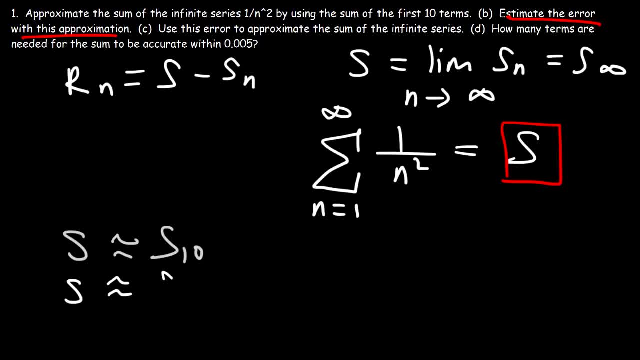 But let's say, if you were to increase n, let's say to 100, s sub 10 would be a better approximation to s than s sub 10.. But if you increase it even more, let's say to a thousand, it's going to be even better. 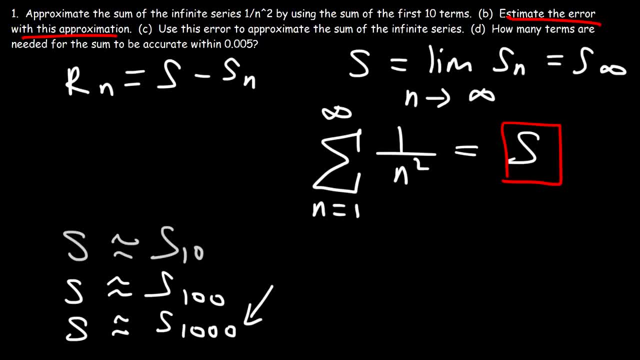 But we don't want to plug in a thousand terms. That's just going to take too long to get the answer. So we want to find a better way to approximate the value of that expression. Now let's add sn to both sides of that equation. 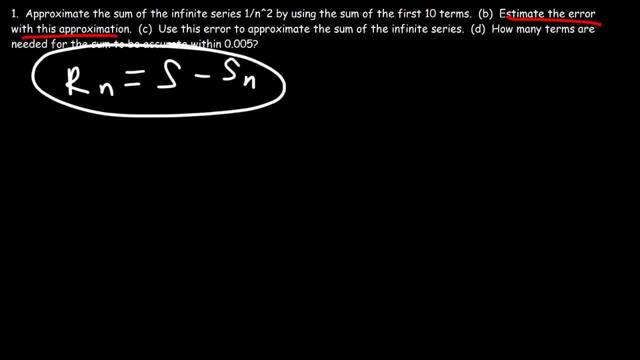 So rn plus sn, that should equal s. Now we know that rn is between these two integrals. So what I'm going to do at this point is I'm going to add sn to both sides of that, sideways, Because I'm going to be incorporating it into stichERS after stich is complicated. 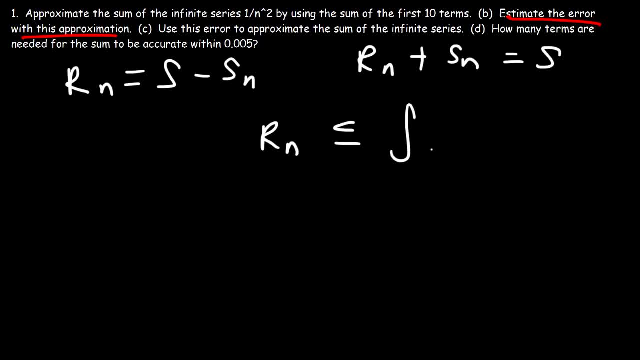 So I'm going to take my integer here. So what I'm going to do at this point is I'm going to add s sub n to each side of this expression. So then I'm going to get this s sub n plus this integral. 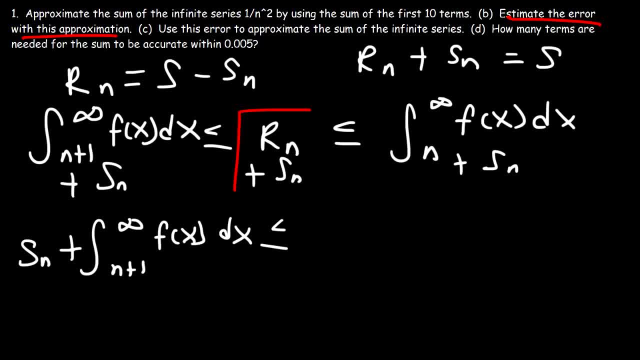 That's going to be less than or equal to, and then I can replace this with s, because s is rn plus sn. What this is going to give me is it's going to give me a range for the sum of the infinite series, which is what I want for part c. 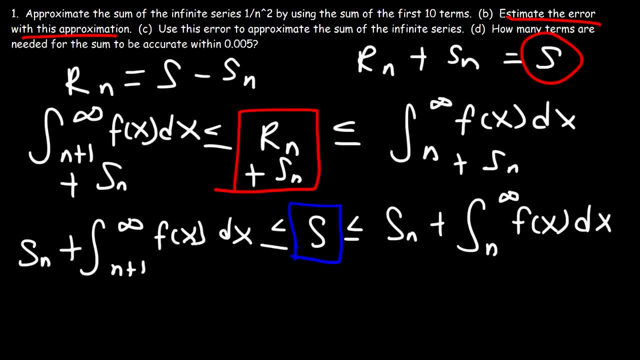 Now n is 10 for this example, so this is going to be s10, and when n is 10,, this is 0. It's going to be well, right now I'm going to write it as 1 over n plus 1, and this was. 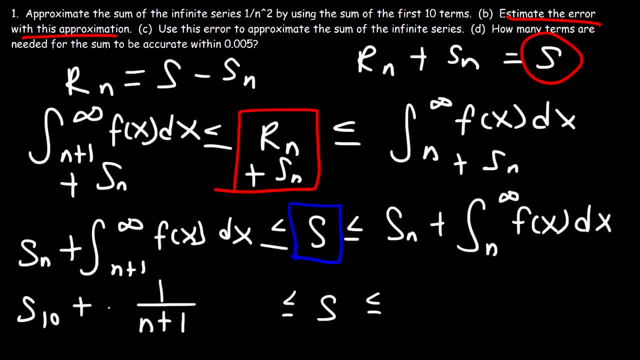 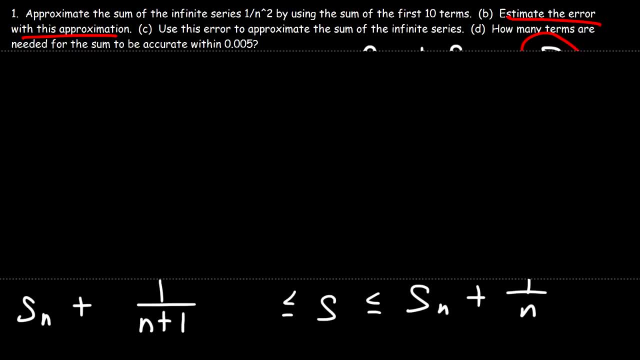 1 over n, So let me keep it in terms of n for now. So I have s sub n plus 1 over n plus 1, and then s sub n plus 1 over n, So n is 10, and this is going to give us this for now. 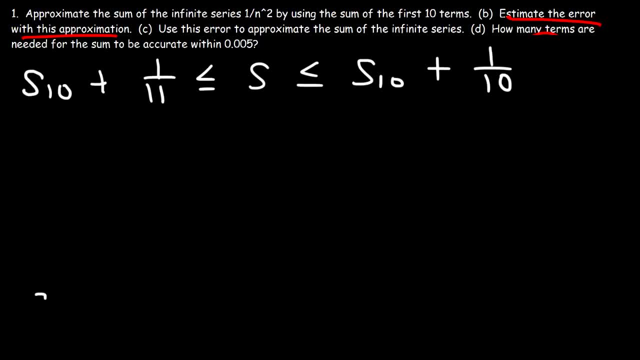 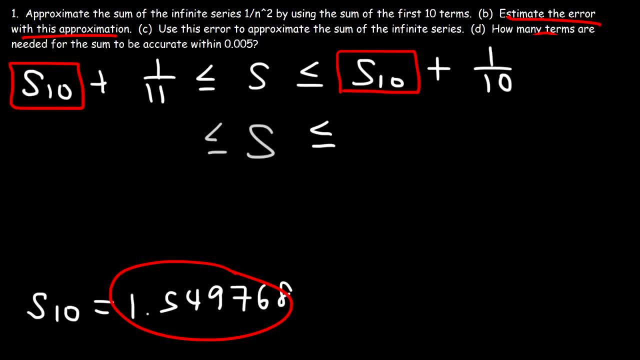 So 1.549768 plus 1 over 11,, that's going to be 1.6406771.. And then 1.549768 plus 1 over 10,, that's going to be 1.649768.. 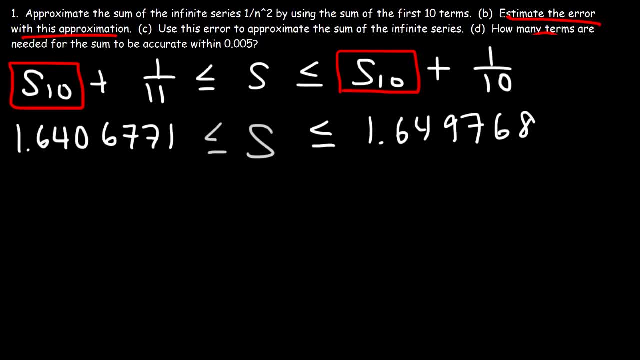 So the true sum is somewhere between these two values. Now let's say, if you were to take a calculator- it could be a scientific calculator or a graphing calculator- and plug this in. Hopefully you have this function. Let's calculate S100.. 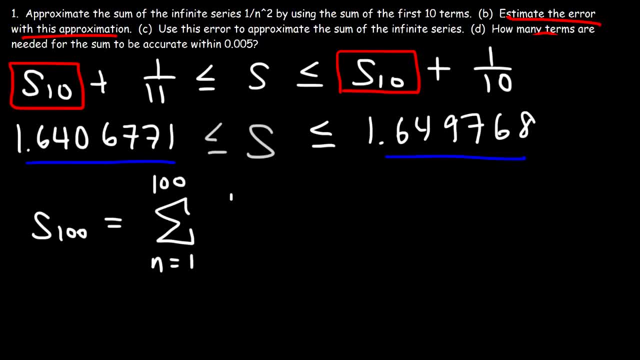 So we're going to go from 1 to 100, and we're going to just add up the terms, the first 100 terms. If you plug this into your calculator, you should get 1.6349839.. So notice the difference between S sub 10 and S sub 100. 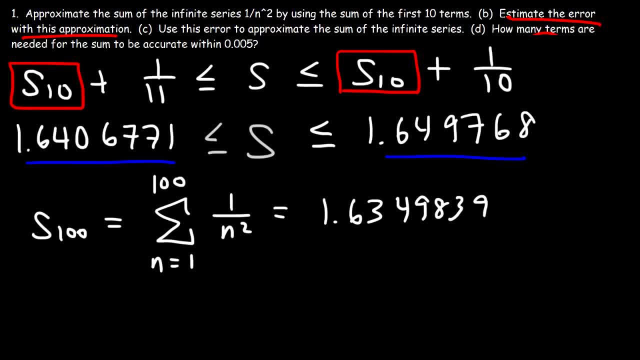 S10 was 1.549768, S100 is 1.6349839, it's higher, but if we go even higher- let's say if n goes to 1,000, then it should give us a more accurate result. 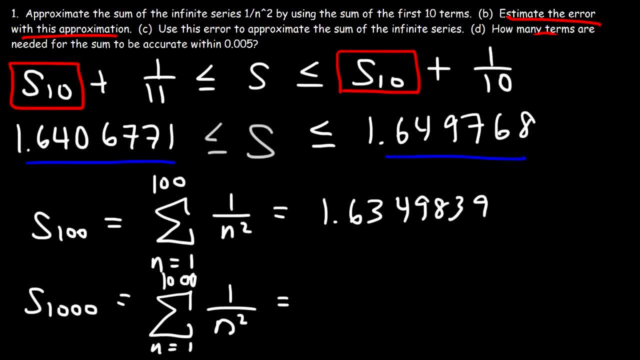 So make sure to use a calculator for this. This might take a hot minute for this one to add the first 1,000 terms. You should get this answer- at least that's what I got- And notice that this answer is greater than 1.6406771, but less than this number. 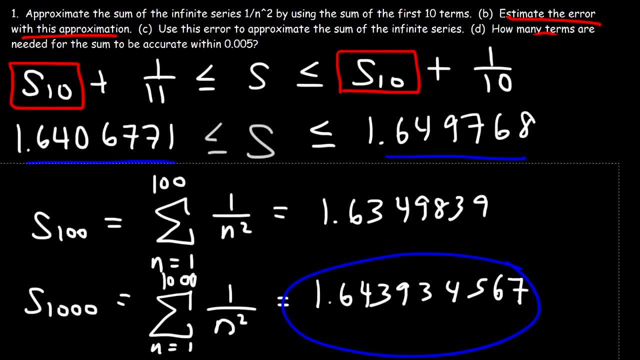 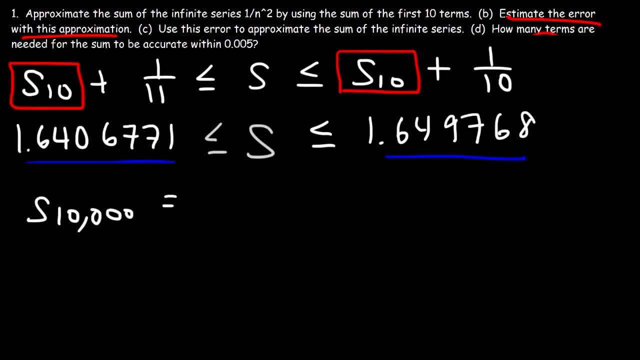 And I tried it one more time. so I went up to 1,000, and it took a few minutes for my calculator to get the answer. I mean I went up to 10,000,. I mean I think it took like 5 to 10 minutes. 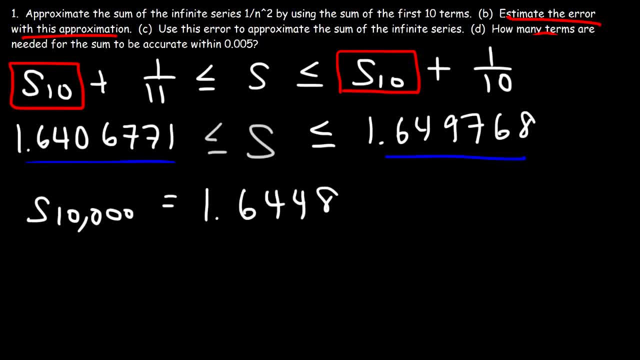 And it was 1.644.. That's what I got. That's what I got, So I subtract out for whatever I get from our economic guide. Now again, I've got it all across this sum set And I heart coded this sum set. 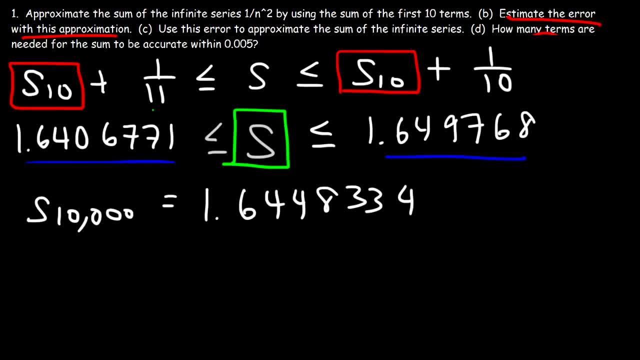 S10 is 1. 25, and s10 is 1.6, I can dump the visit in. I can dump se for 1, 200, because for 1.6, we cannot multiply our profit. kostim and Nья weights. 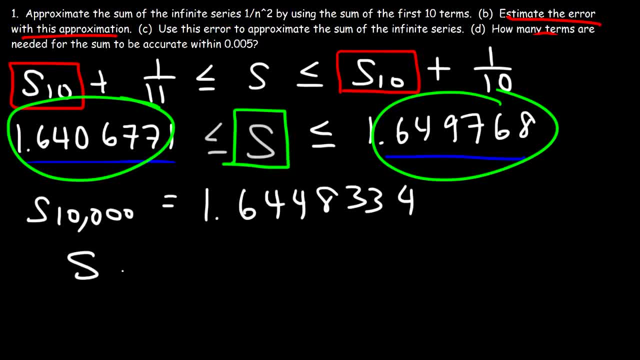 Now, in order to build our profit, I need S10.. You can simply use your math. This form has values that go with ?1, instead of 2 and P atge 3.. excellent For these. if you're a hard worker, don't know. there is a direction here. 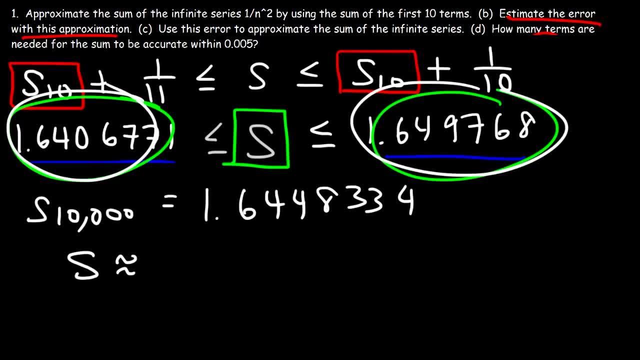 You don't know the direction, so don't guess, because I told you. All right, those two numbers. so let's take one point six, four, zero, six, seven, seven, one, and add it to one point six, four, nine, seven, six, eight. so add them, and then 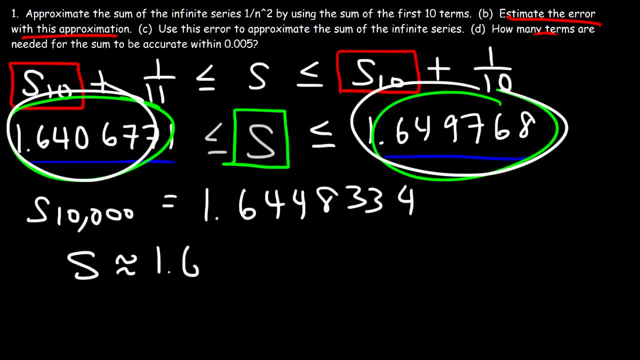 divide by two, and you should get this number one point six, four, five, two, and so the actual sum should be somewhat close to this value. if we just average these two numbers- and we can see that these two numbers aren't too far apart- they both round to one point six, four, five, and so that's a good approximation. 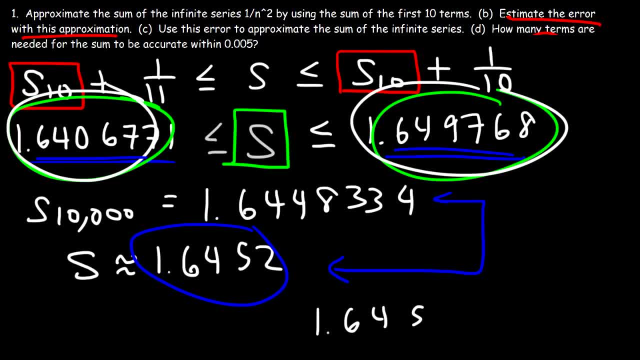 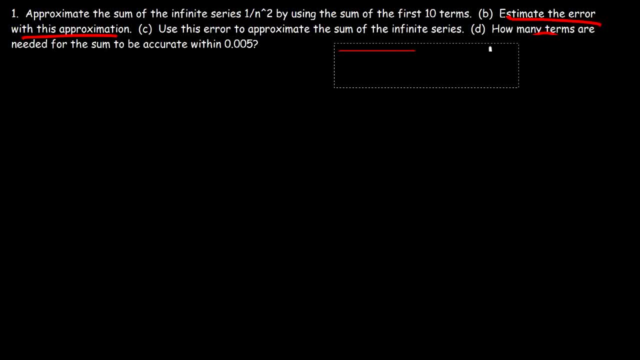 of the sum of the infinite series. now let's move on to part d. how many terms are needed for the sum to be accurate? within 0.05? so the remainder estimate is at most the integral from n to infinity of x, DX, which we found out to be one. 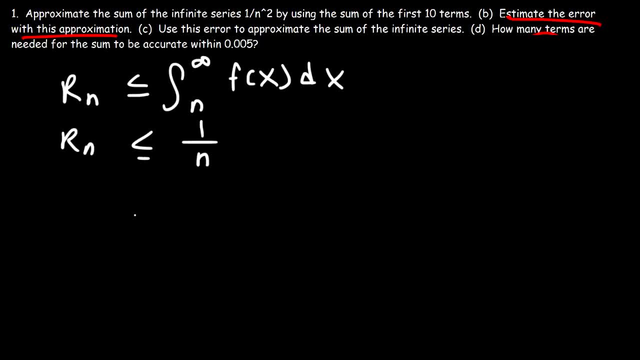 over n in this problem, and so we said that r sub 10 was less than equal to 0.1. but now, this time, we want the sum to be accurate within 0.005 and we're looking for the number of terms. so basically, we're looking for n when r sub. 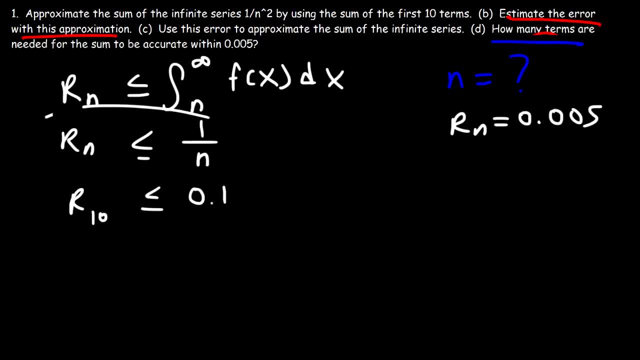 n is 0.005, so we need to use this expression. so let's replace r sub n with this number. so we're going to have: 0.005 is less than or equal to 1 over n. now what we're going to do is raise both sides to the negative one, so 1 over.